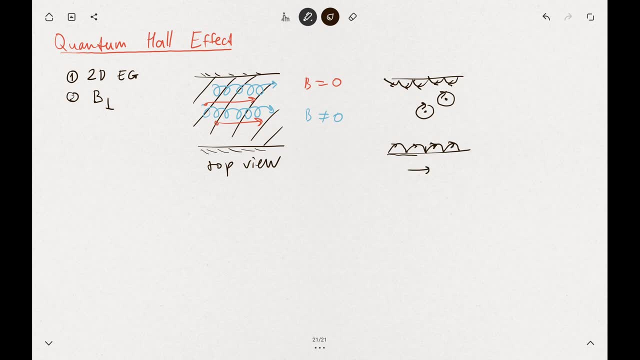 bottom edge, you will have the right propagating mode, You have these right moving electrons, And on the top edge you have the left moving electrons. So you have now, very naively speaking, you have one-dimensional channels, those two one-dimensional channels, And the behavior along those edges has a 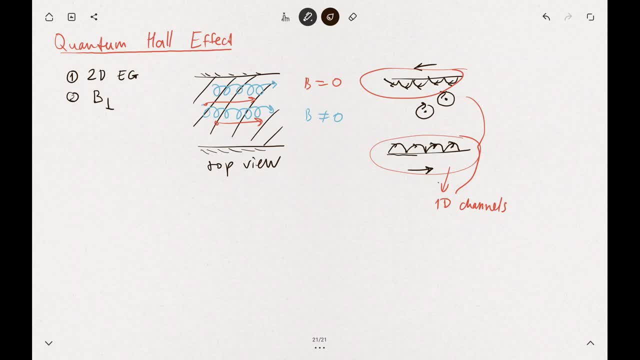 chirality right, So there's right moving and left moving particles. So those edges they are chiral edges And it's quite a nice system to study the quantum Hall effect. So you start from a two-dimensional system, Then the bulk. 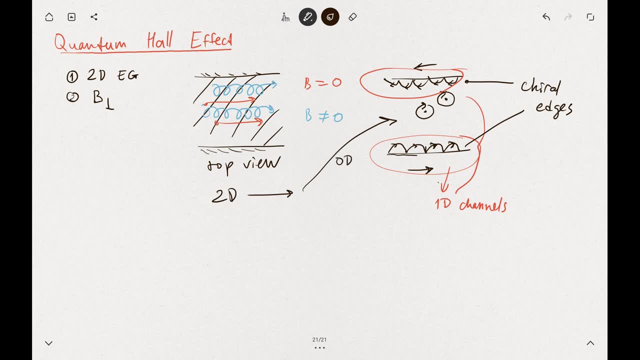 essentially becomes zero-dimensional, So all the motion stops and only localizes around these small cyclotron orbits And you would also have 1d channels. So in this system you can study both two- dimensions, 1-dimensional and zero-dimensional systems. To go beyond this kind of 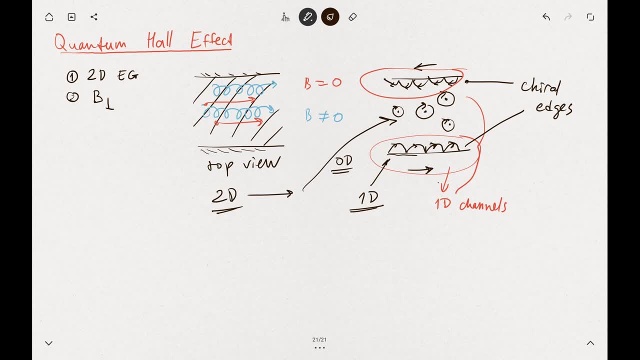 of simplified picture. we should, we should, treat the problem quantum mechanically. so, in addition to this semi-classical description of the cyclotron orbits and the skipping skipping of those orbits on the edges, we can do a better job by considering the quantum mechanics, and and for this we would need to introduce the concept of landau levels. 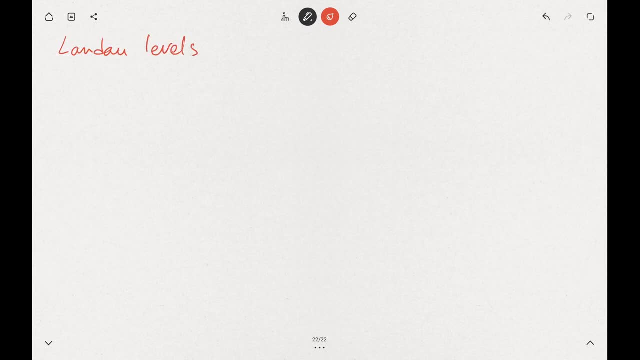 so how do we do this and what? what are those landau levels? you would need to have um to add the magnetic field to quantum mechanics and the conventional way to do it is to use a vector potential. so the magnetic field, just to remind you, the magnetic field is the- is the curl of the vector. 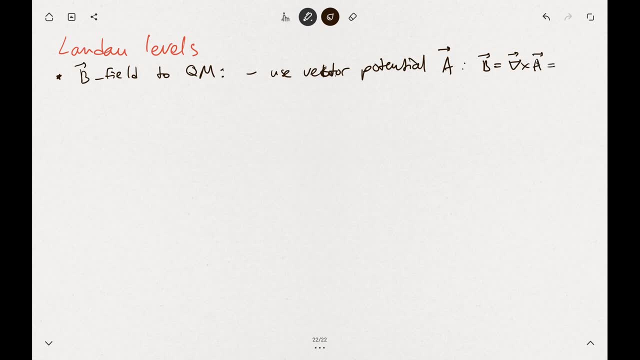 potential, and in our case it's a magnitude of the field times in the in the z direction, because it's a perpendicular to the plane. so then you can write the hamiltonian. so you can write the hamiltonian in this form: minus e a squared. 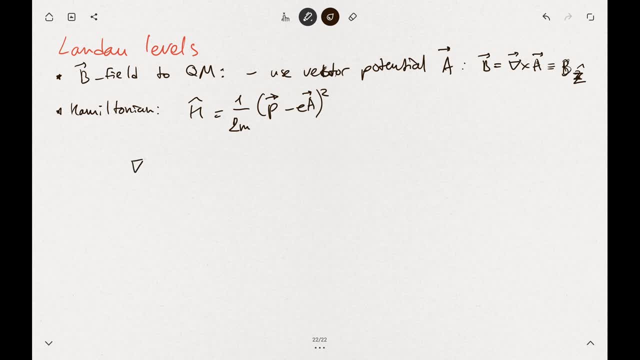 so now we have this interesting term because the magnetic field is is the curl of the vector potential, so you can choose a vector potential in multiple ways and it's kind of it's the gauge invariance problem and i think you probably are familiar with this. 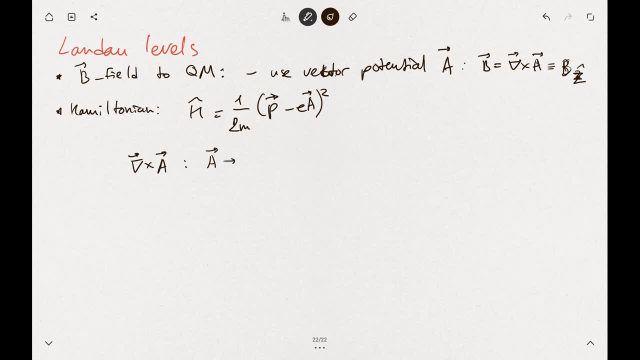 one. so the vector potential. we can introduce instead of this vector potential some other vector potential which is defined as the initial vector potential, plus some function which is a gradient. basically so it's a function which is a gradient of some function, and then you will have this term if you want to look for what happens when you. 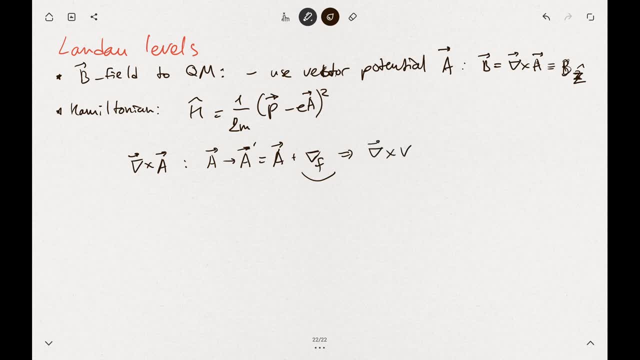 when you take the curl you will have this kind of this term and the curl of the gradient is zero. so any arbitrary function which is a gradient of a function can be added and this is known as the gauge invariance. so this means we can select vector potential multiple in multiple ways. 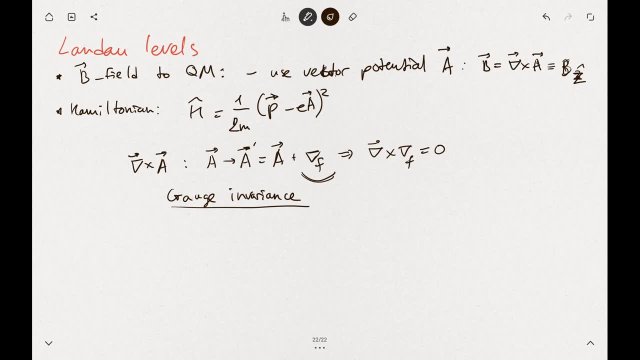 and there are several ways of doing this. there's some, there's symmetric gauge. in this case we will use a Landau gauge which is defined as magnetic field, X direction and J component of the spatial dimension. so in the vector column form you will have it like that. so we can now write down the Schrodinger equation. 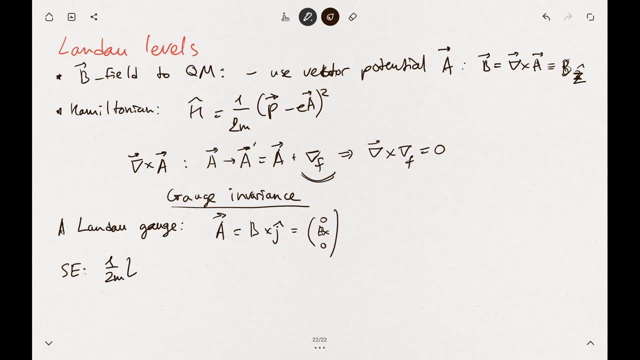 which will be 1 over 2m px squared, and I'm just plugging the vector potential. result: now you have py minus e, b, e, b, x squared, acting on a wave function of Psi. that will be our Schrodinger equation, and note that the vector potential 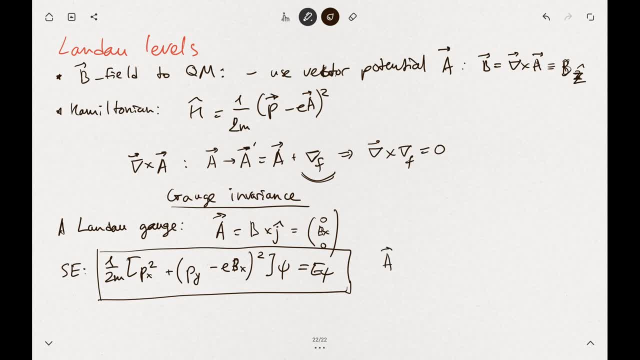 doesn't depend on y, so the a doesn't depend on y and this means we can guess. we can guess of a function in the form of plane wave of y and maybe some unknown function of x, so the wave function, which is a function of both spatial coordinates, x and y. 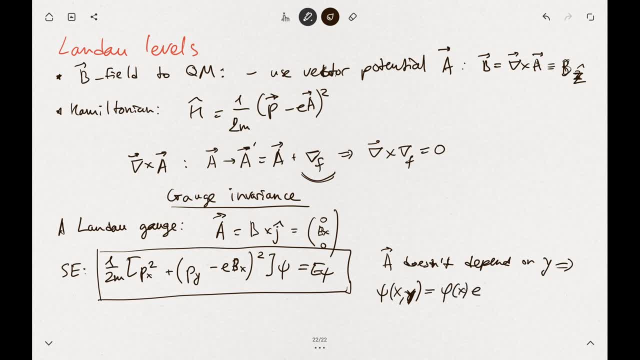 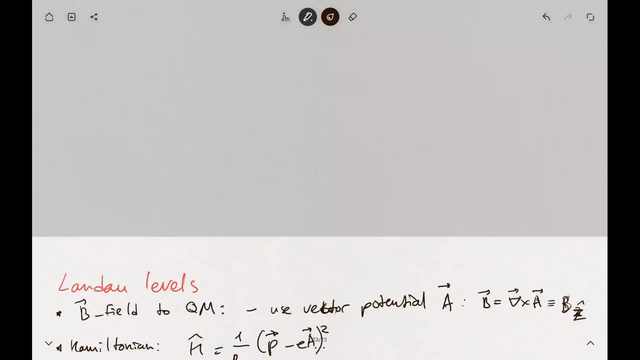 is a sum, unknown function of x coordinate times, the e to the i, k, y, to introduce the plane wave in the y direction. now let's see what happens if we act by the py on on the wave function we get. we get the following: minus i, h, bar, d, d, y, e, i, k. 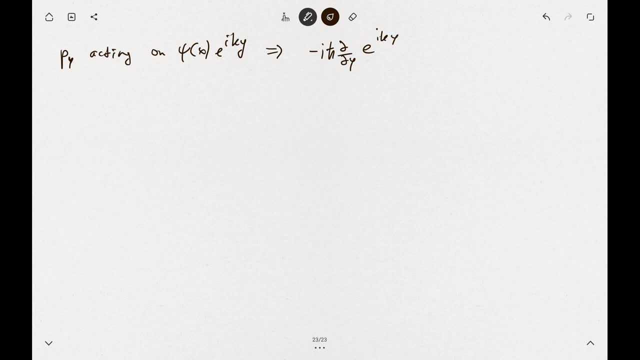 e, i k, y, that's the, that's the py operator acting on a wave function. so basically, on the on the plane wave part, it will result in adding the h bar k. so you have the h bar, the k comes out, i, i k comes out, and minus i i cancel. so you get h bar k. 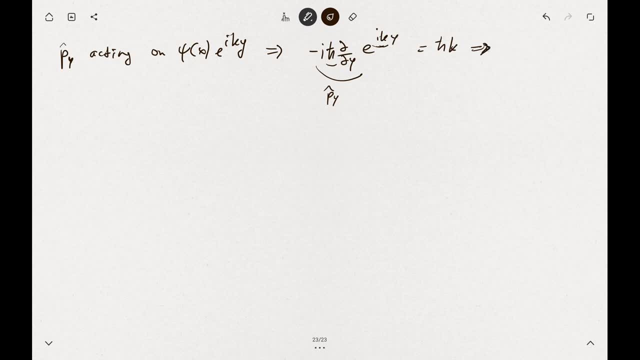 and we can rewrite the hamiltonian using this, this part. so we will have. we have the following: the following hamiltonian, which will now have only y, only x dependence. there's only x dependence. it's p x squared over 12 plus um. let's see: 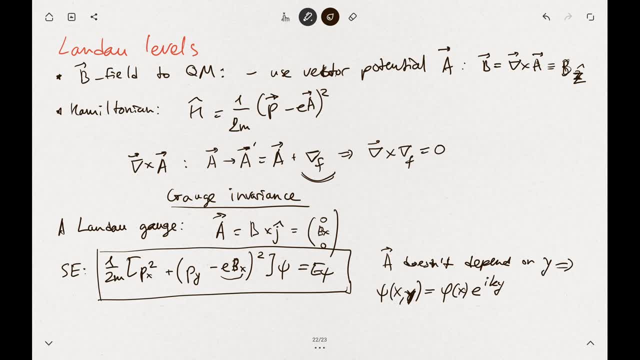 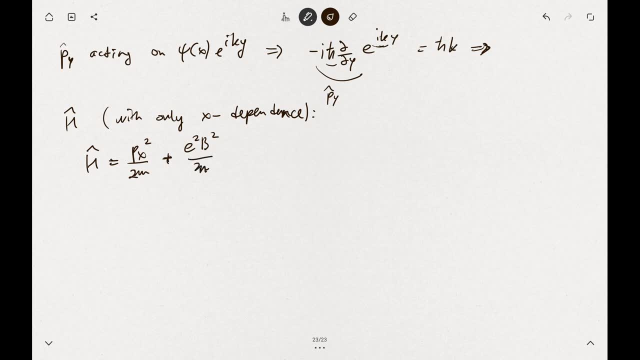 so we have e b x here and we can write it in the form of e square b, square over 2m, and then we have the our result of h bar k. so this one will have a form of x, all other parts minus h bar k over e b. 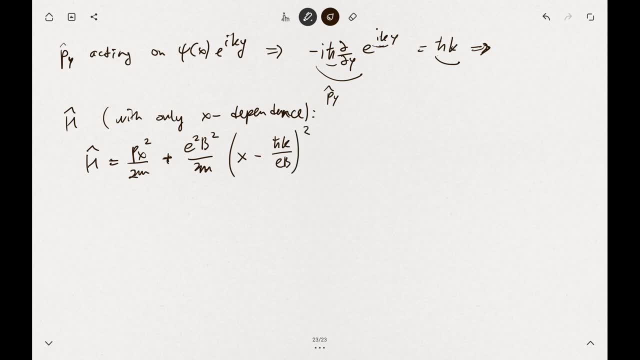 squared and and the minus is from the sine of the electron charge. so if you look at this one, this is the. basically, this one is the hamiltonian of the one-dimensional harmonic oscillator, 1d harmonic oscillator and you can just say that the wave functions are centered at some uh. so this is our. 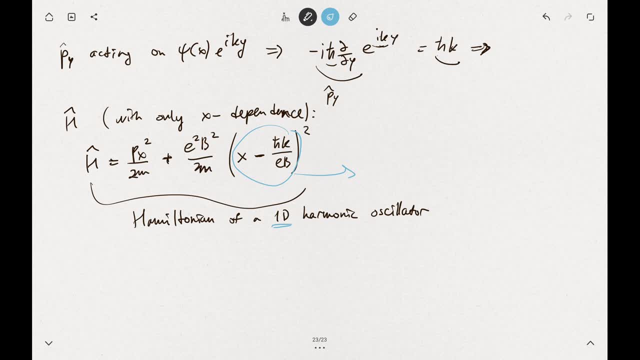 this is our um x component. so this is one dimension. so it's on the x component there and you can say that this um, the center of the wave function, would be at this x, 0, which are h bar h bar k over e b. so the wave functions are centered. wave functions are centered at x, naught and this k. 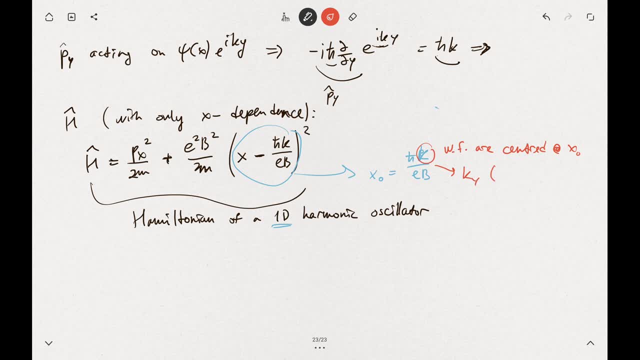 is actually is ky for motion in y direction. so those are plane waves, as we discussed just a few minutes ago. for motion in y direction we can compare them, um to the motion when wave is moderating. sometimes in the literature you can find um these this term: h bar over e b, a square root actually of h bar over e b. 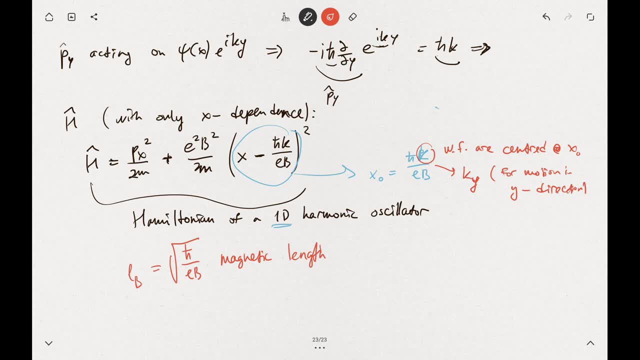 which is defined as the magnetic lens, a dimension of the problem. so basically, it kind of tells you what would be the, what would be the size of the of the wave function. all right, so we have a Schrodinger equation. we know it's the, it's the one-dimensional harmonic.